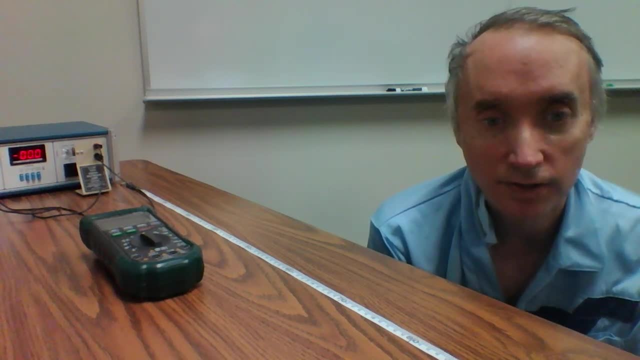 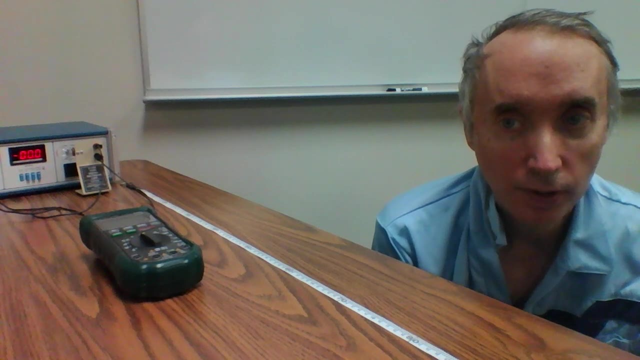 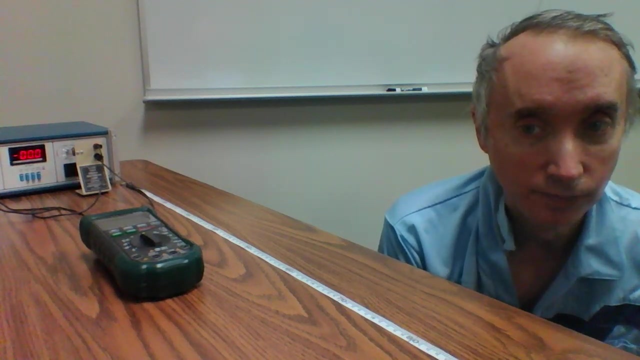 So, on the Microsoft Excel worksheet, click on the tab at the bottom of the worksheet that says 13 Photometry. So what we want to be able to do is to mathematically come up with a formula that is going to relate the actual brightness of a light bulb, which is going to be its luminosity L, to its apparent brightness, which is going to be F. 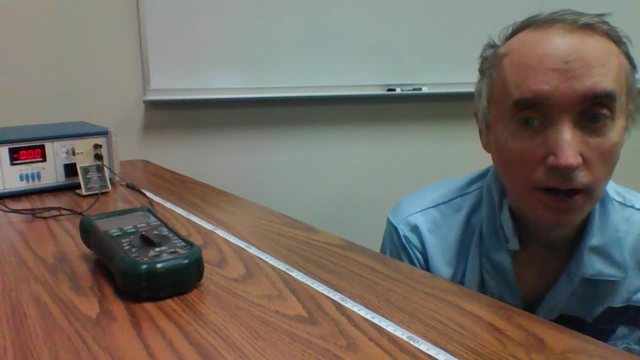 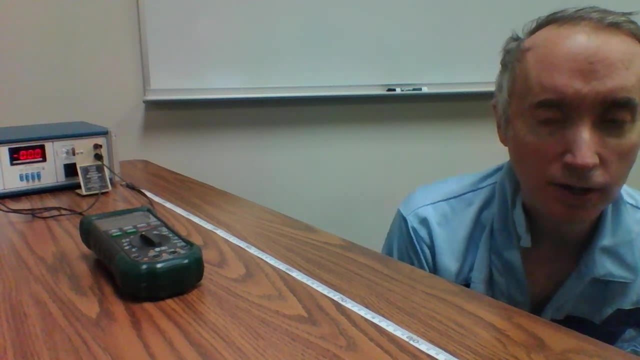 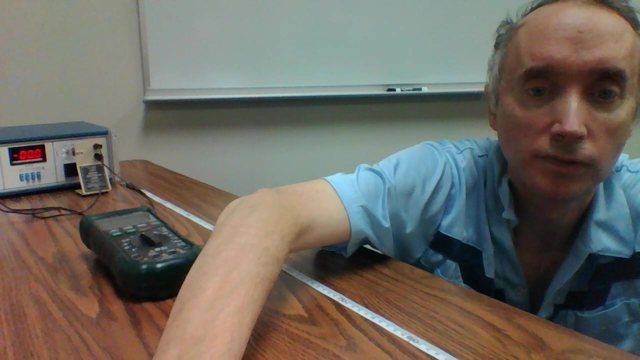 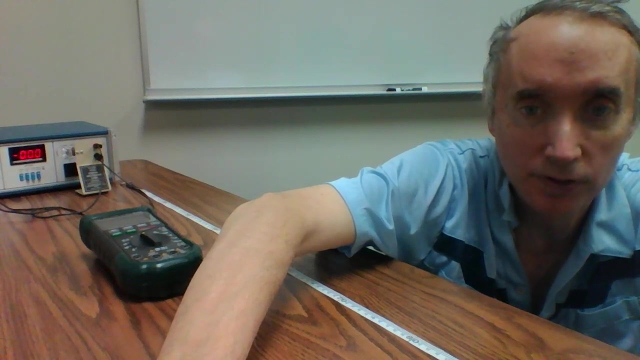 For energy flux And then also the distance. So how far away is the light bulb? So here, next let's do the pre-lab. So what's the purpose of the lab? So go down into the lab to where it says Purpose, and then copy and paste it there, The safety instructions for it. 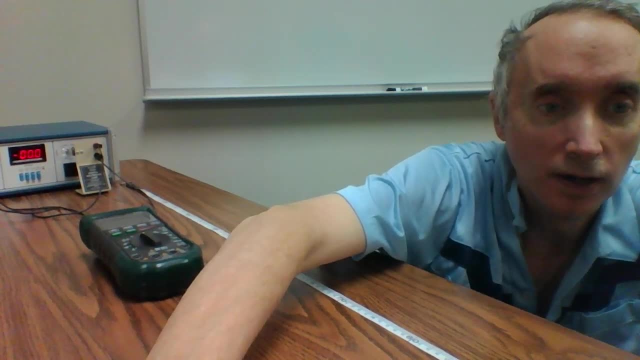 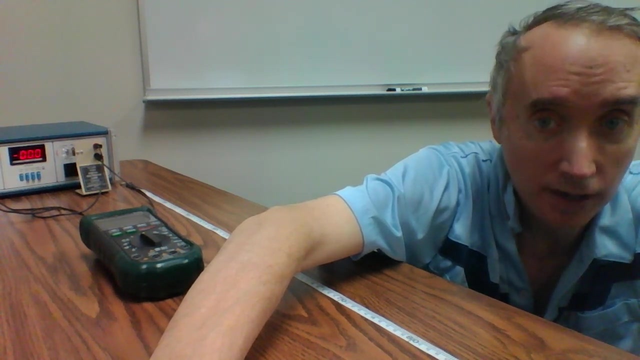 So go ahead and copy and paste those. What is apparent brightness? So you should write down what the letter for apparent brightness is and then explain it. Number 4, if you're walking away from a light bulb, the light bulb's apparent brightness will it increase, will it decrease or will it be the same? So just highlight one of those three answers. 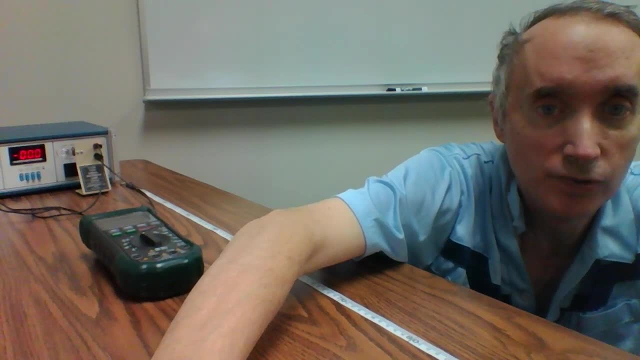 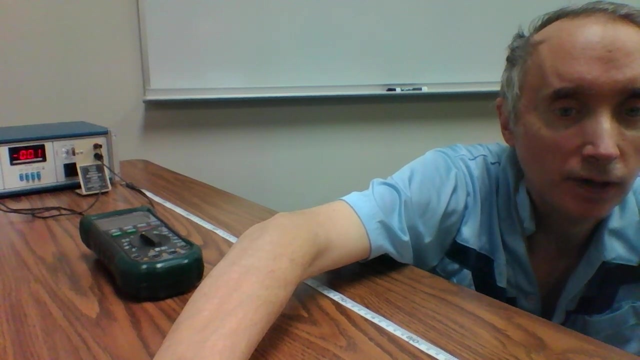 Okay, question number five: what's the device that will be used to measure the apparent brightness? So that is down in the lab, Okay, Okay. so now let's go down into the procedure. Okay, And you'll see that it. 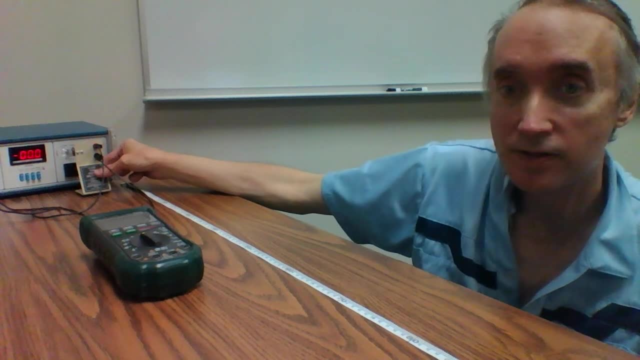 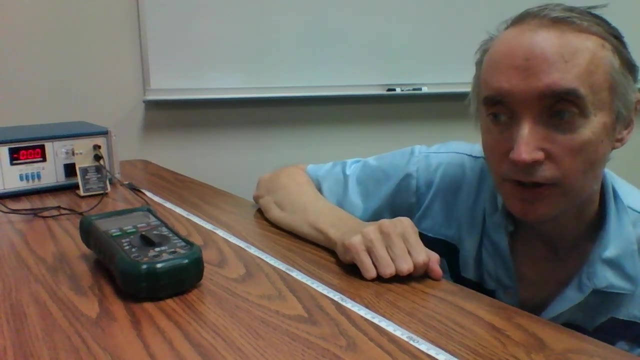 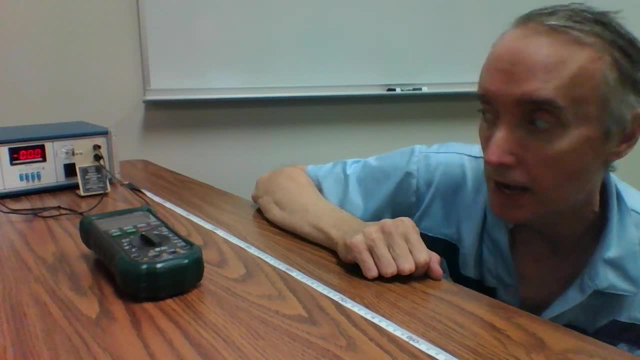 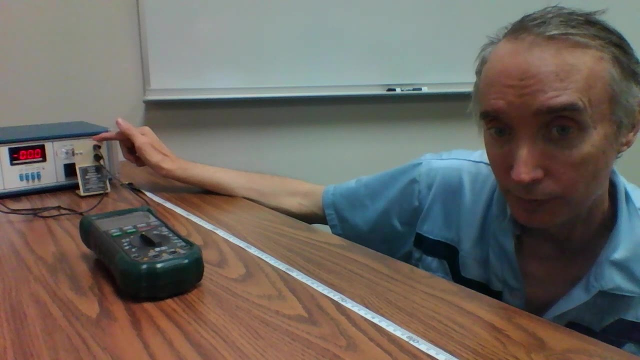 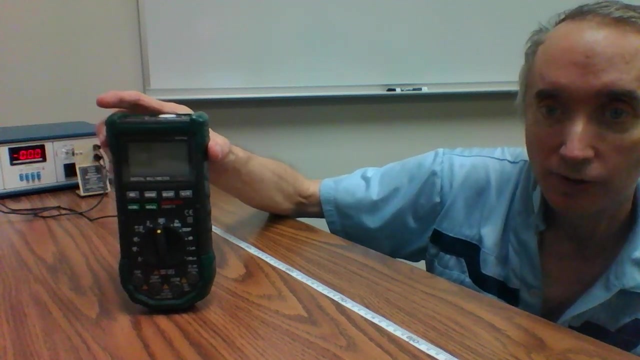 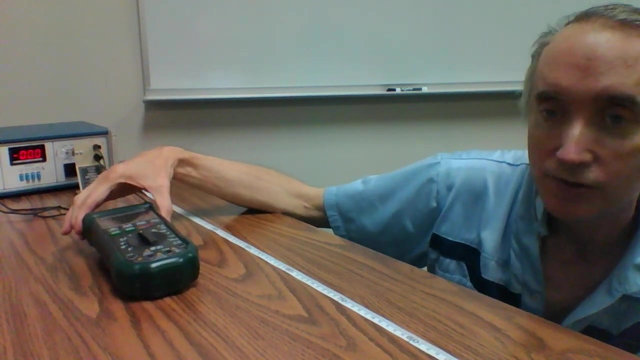 a certain brightness. So the actual brightness is going to be L, and then what we're going to be doing is measuring the apparent brightness of the light bulb with our photometer, which I'm going to try to use, this multimeter. So this has a built in photometer and we're going to use that to measure the brightness. 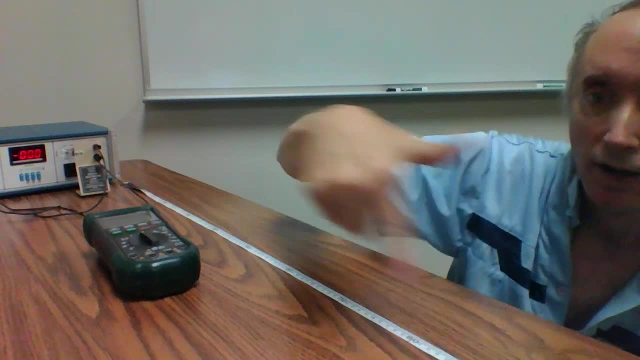 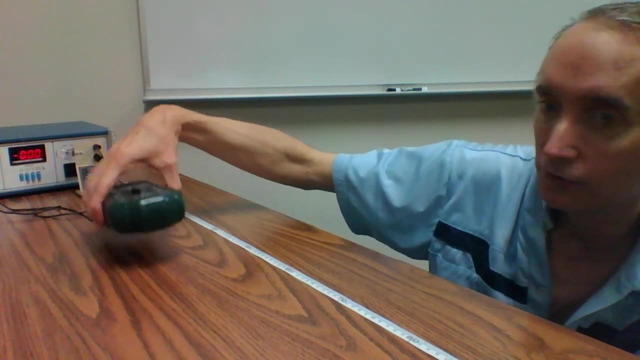 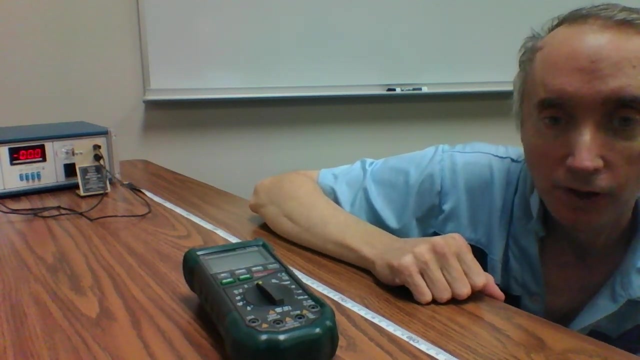 of the light bulb. and then I've got here, I have a measuring tape and we're going to also, we're going to measure the brightness at different distances away from the light bulb, and what I'm going to do is I'm going to give you those numbers and then you're going to put them. 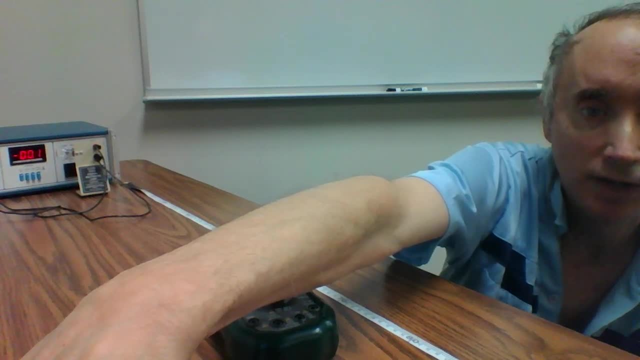 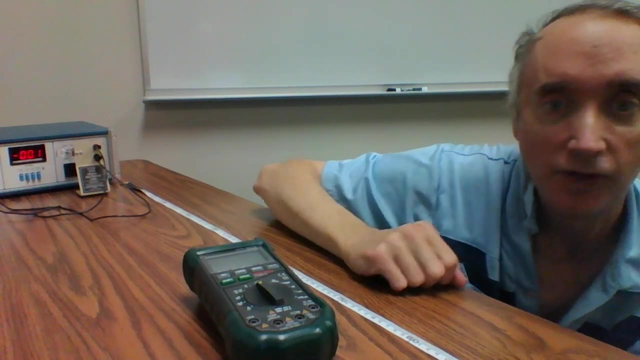 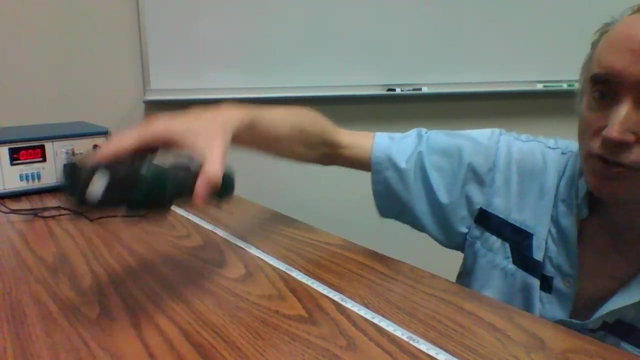 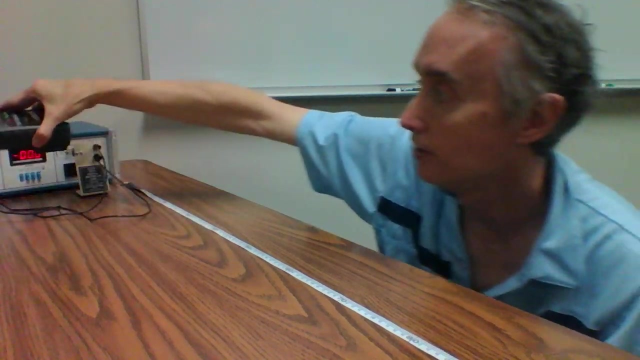 in the light bulb. Now you'll notice that in the original procedure in the lab it says to measure the brightness from five different directions. so originally the lab calls for measuring the brightness in this direction and then measuring the brightness in that direction and then measuring it at 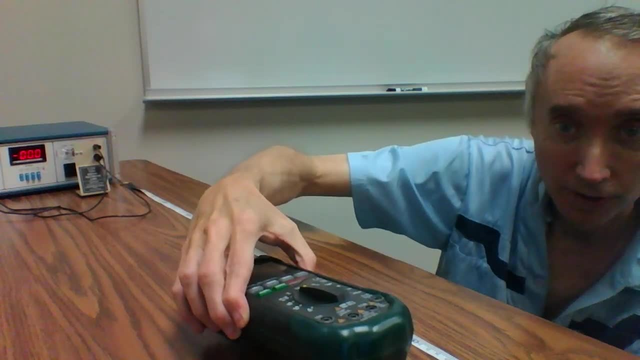 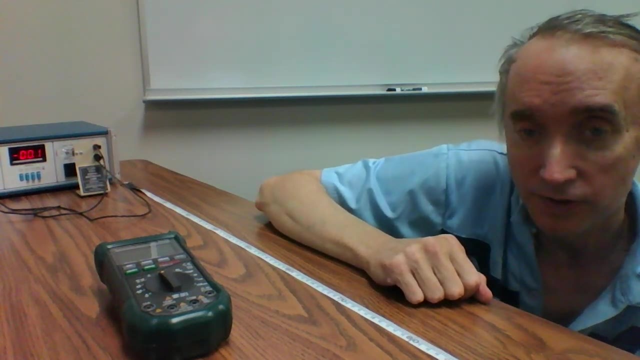 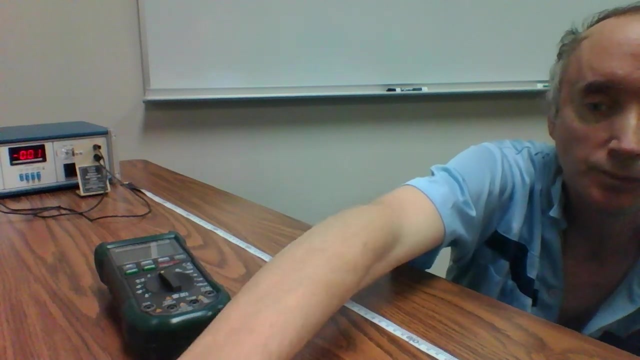 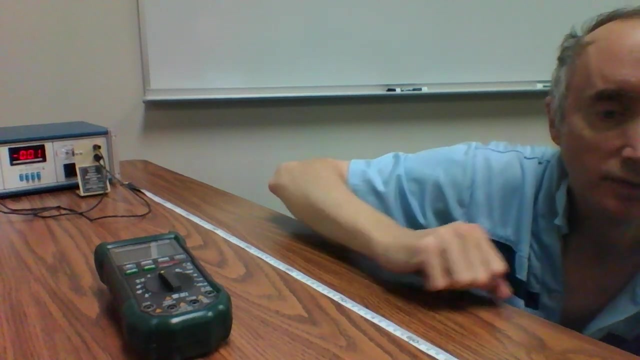 angles And then perpendicular. So perpendicular would be number three. What we're going to do is only three. So we're going to measure the brightness of the light bulb in that direction only. So if you continue to go down, you'll see there is the data table that you're going to fill. 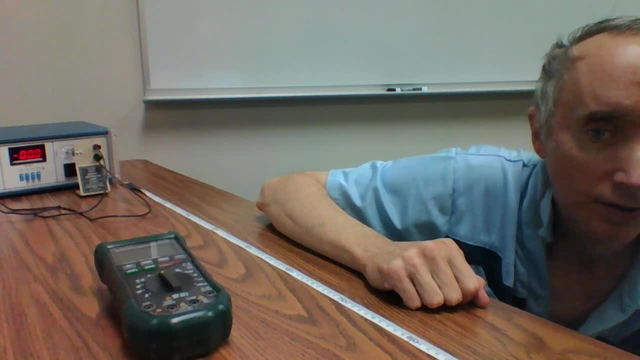 out. I'm only going to fill out column number one. so I'm going to tell you what the distances are and then you're going to put them in the data table and then I will tell you what the readout on the photometer is and you can put that in column, in the column that says number. 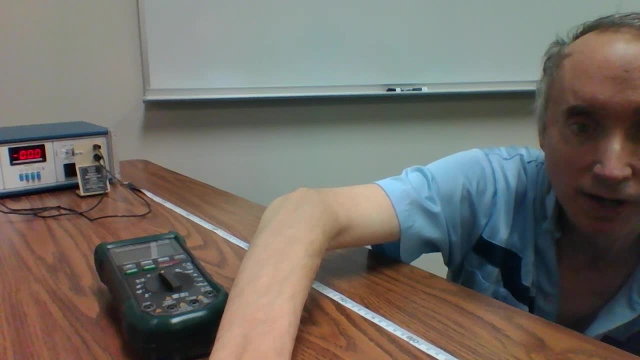 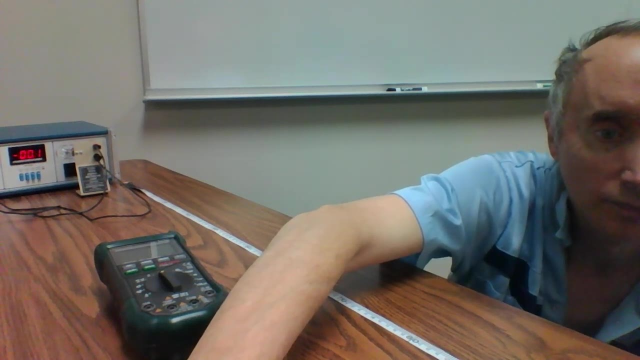 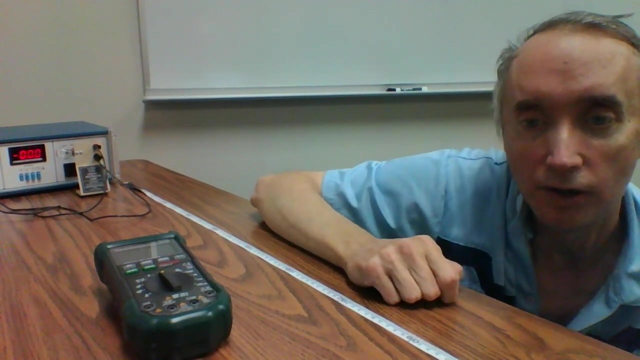 three, or you could just put it in the last column, which says the average. so it doesn't really make any difference Where you put that data. Okay, so I think we're ready now, so I'm going to stop the video here. I'm going to turn out.